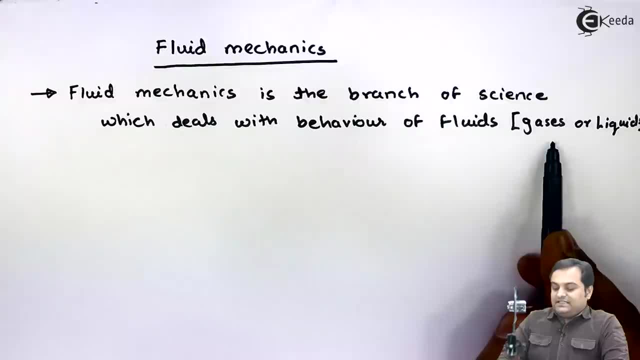 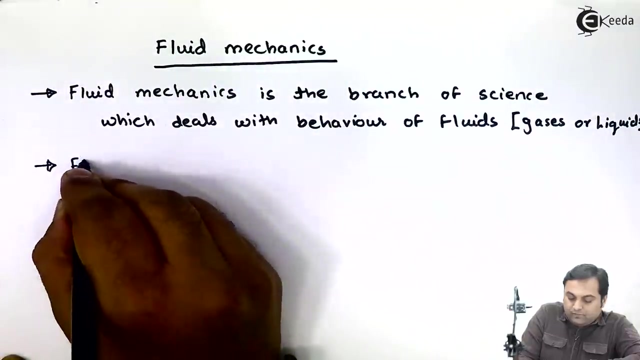 because when we say fluid we mean that gases or liquids. it means fluid doesn't mean that they should only be liquid. gases can also be treated as fluids. so when we are studying the behavior of gases or liquids, that study is called as fluid mechanics. now, in fluid mechanics we can say that fluid mechanics 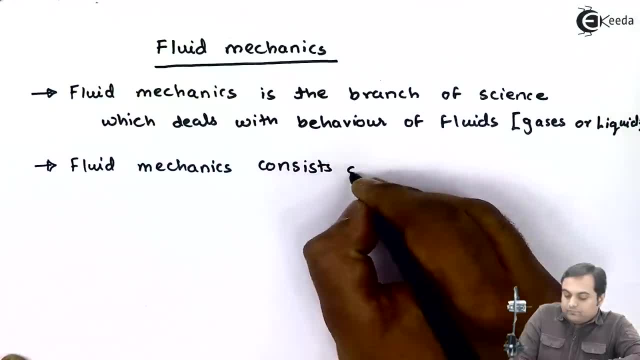 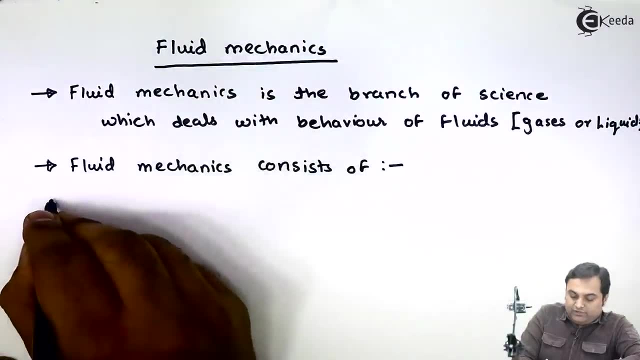 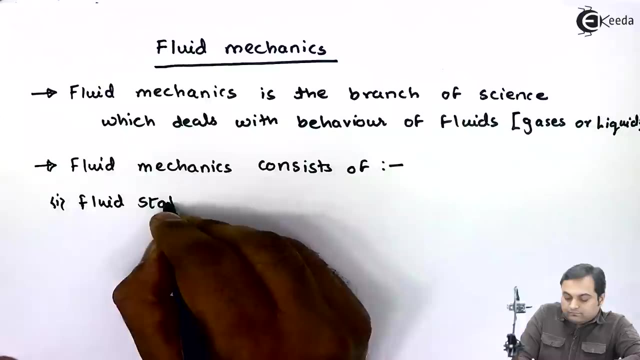 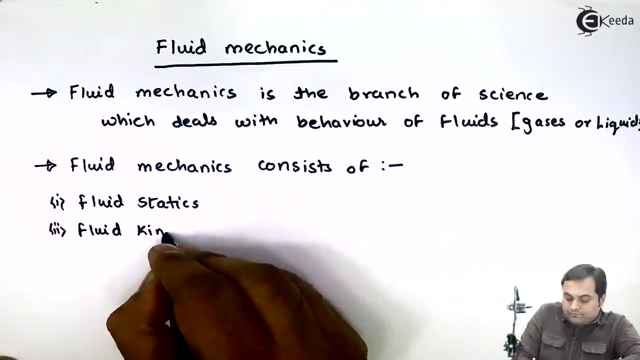 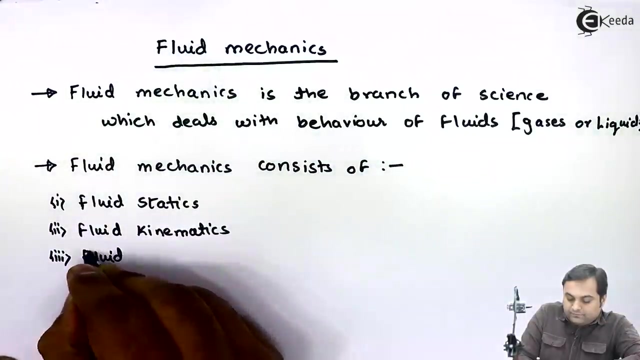 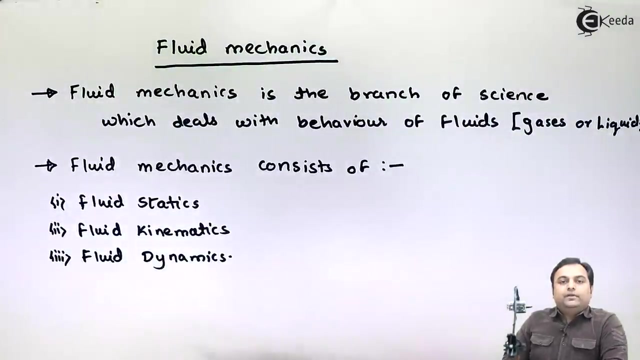 it consists of normally fluid mechanics. it is divided into three parts. those are: number one, fluid statics. second, fluid kinematics and the third one fluid dynamics. so here we have three different parts of fluid mechanics: fluid statics, first part, fluid kinematics the second part, and fluid dynamics, the third part. now when 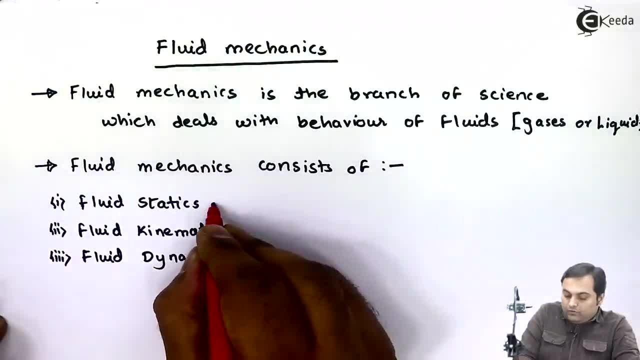 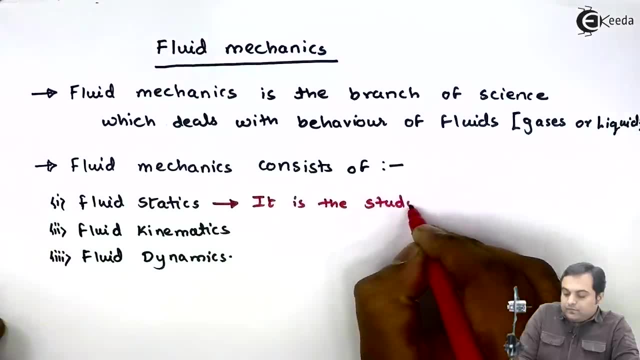 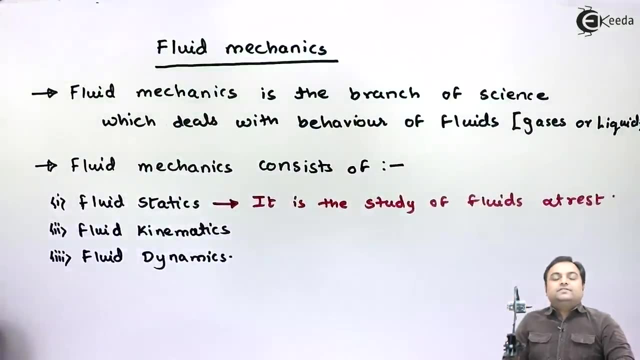 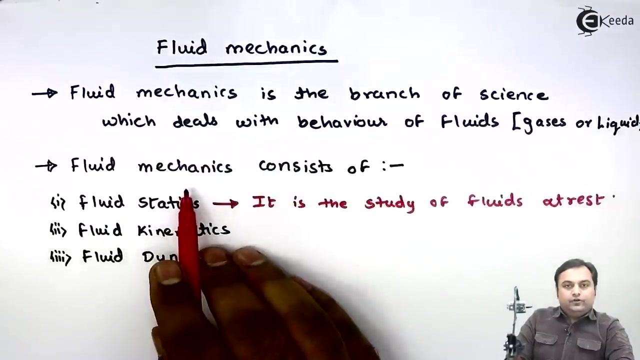 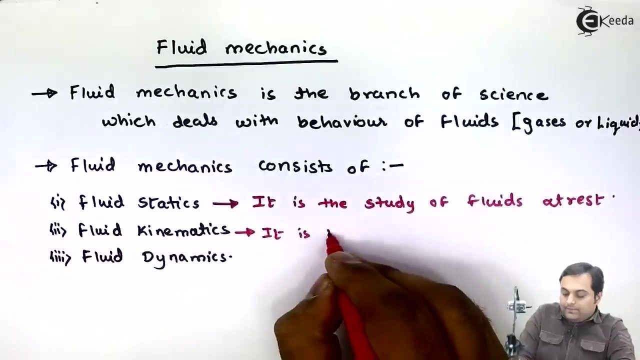 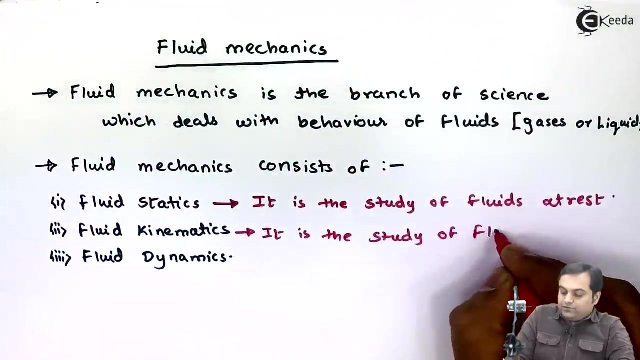 we are talking about fluid statics. fluid statics, it is the study of fluids at rest. so whenever we are studying a fluid which is at rest, it means it becomes fluid statics. that is a branch of fluid mechanics. next, fluid kinematics, it is the study of fluids in motion. 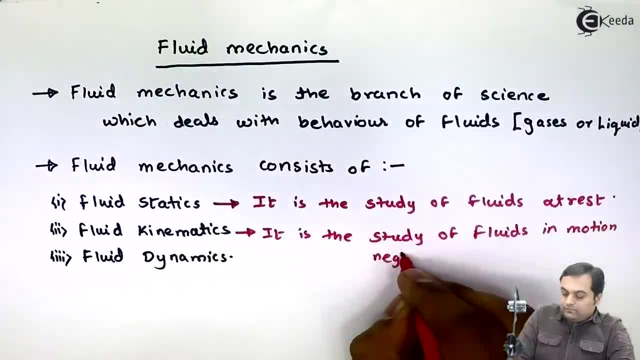 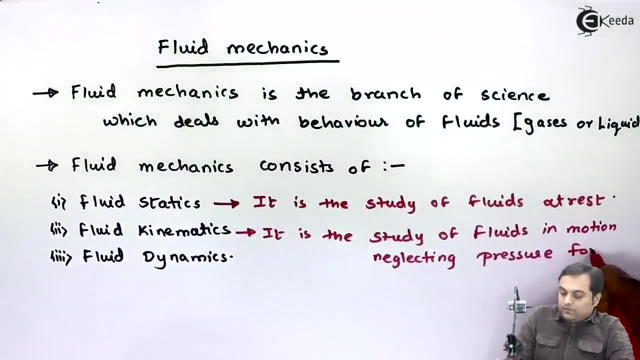 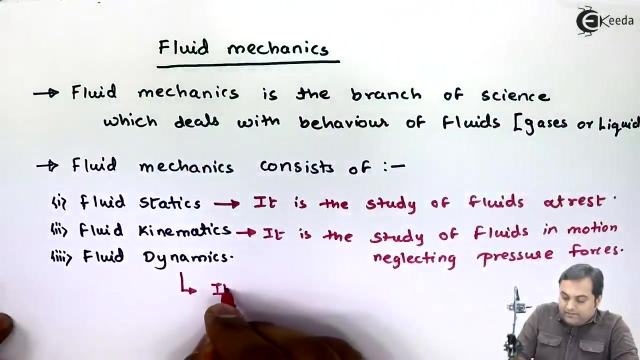 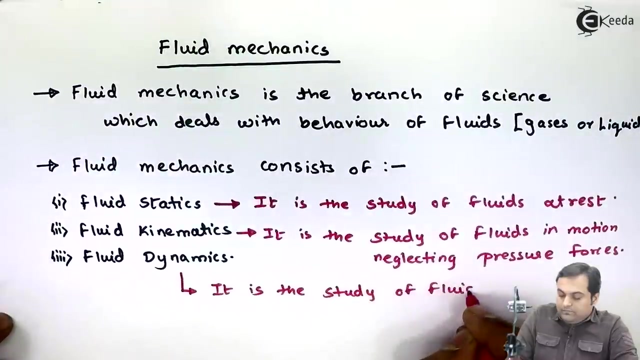 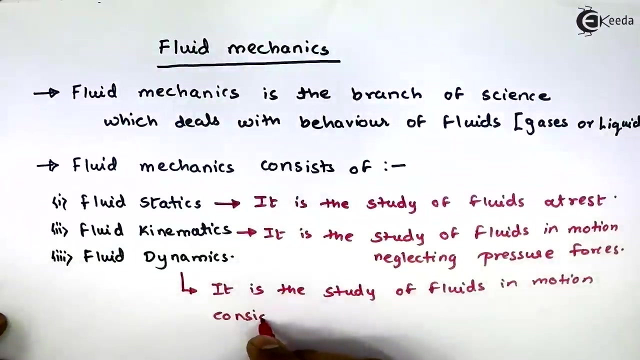 neglecting pressure forces. that is, if we are studying the fluids which are in motion and neglecting the pressure forces, then it becomes fluid kinematics and the last part, that is fluid dynamics. it is the study of fluids in motion considering the pressure forces. so here we have seen that what is?